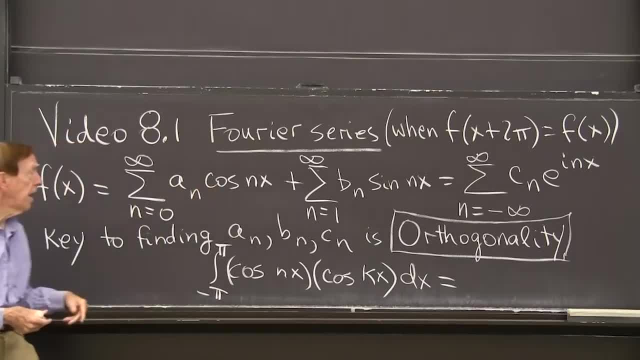 That tells us how much of cosine nx is in the big function f of x. Notice that the cosines start at n equals 0, because cosine of 0 is 1.. So that's a, There's a, There's an a 0 in our sum. 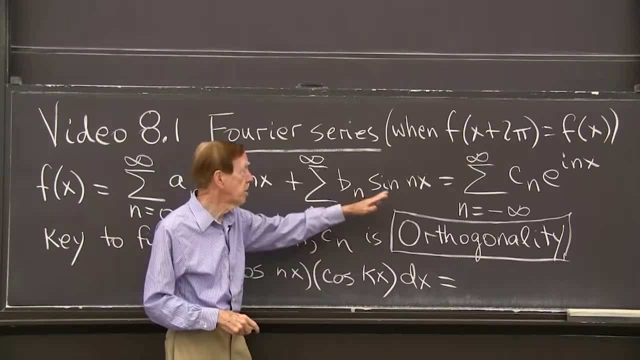 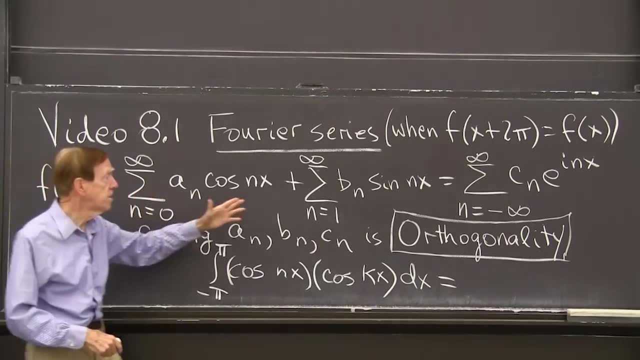 But there isn't a b? 0, because n equals 0. The sine would be 0. And we don't get anything there. So we're looking for the a? n's and b? n's And really I want to show you at the same time. 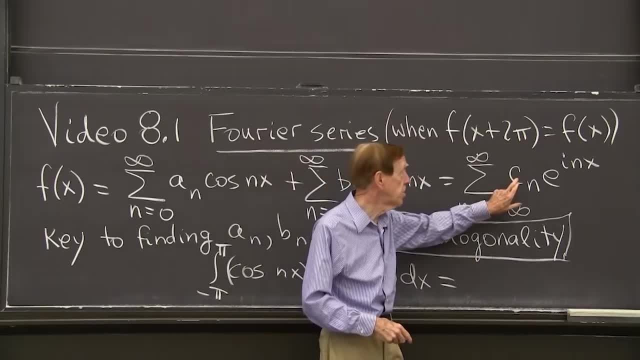 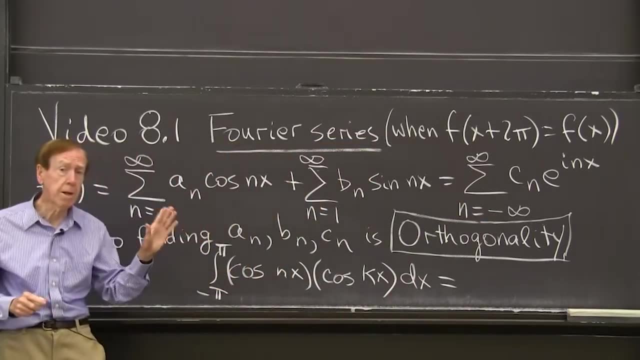 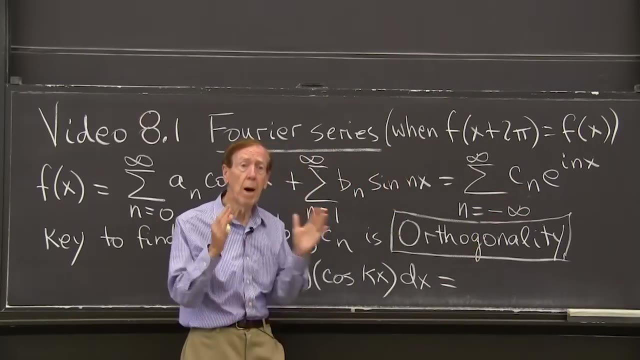 the complex form with coefficient cn And now n goes from minus infinity to infinity. That's really the more beautiful, That's the more beautiful, That's the more beautiful, That's the more beautiful form, because there's a nice formula for cn. that one formula for cn does the job. 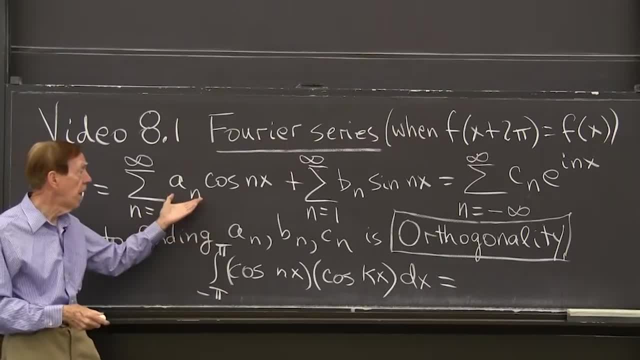 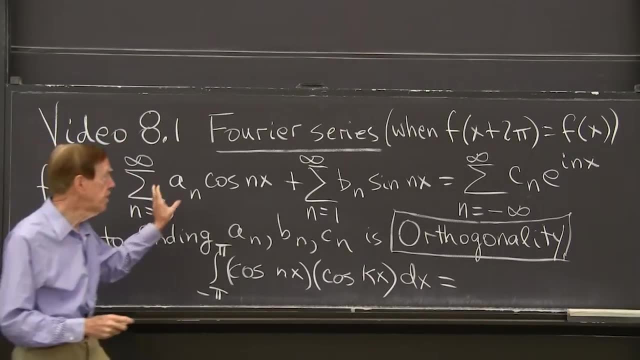 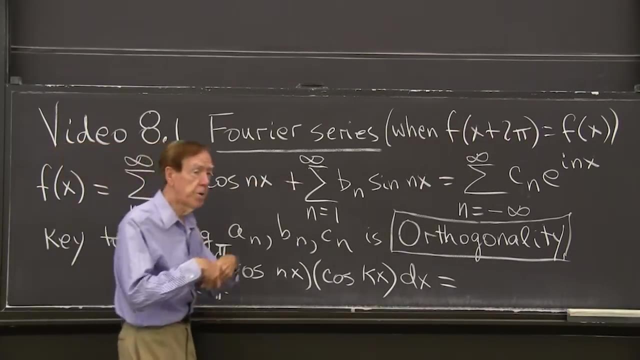 Whereas here I will need a separate formula for a- n and for b n. OK, But so this is like natural, when the function is real. But in the end, and for the discrete Fourier transform and for the fast Fourier transform, the complex case will win. 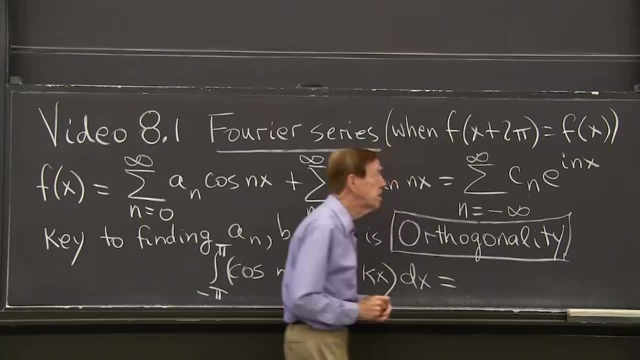 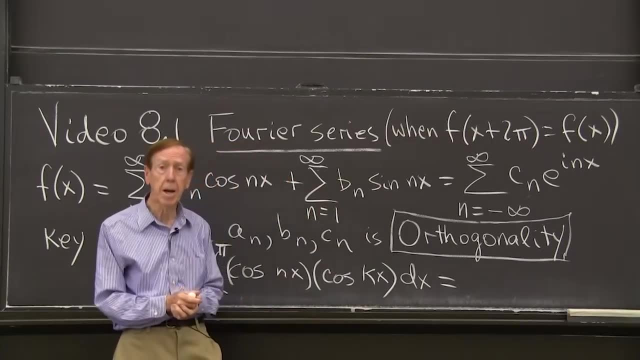 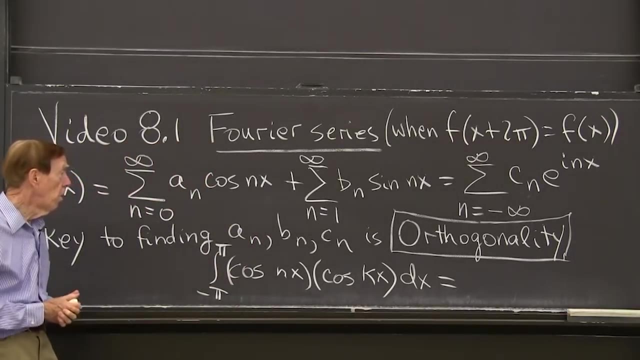 And of course everybody sees that e to the inx by Euler's great formula is a combination of cosine nx and sine nx. So I can use those, or I can use cosines and sines, OK. So how do you find these numbers? 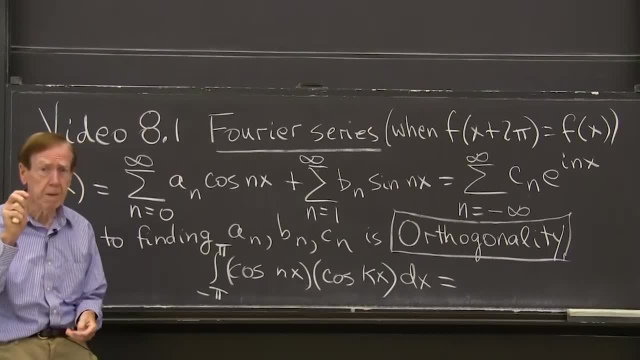 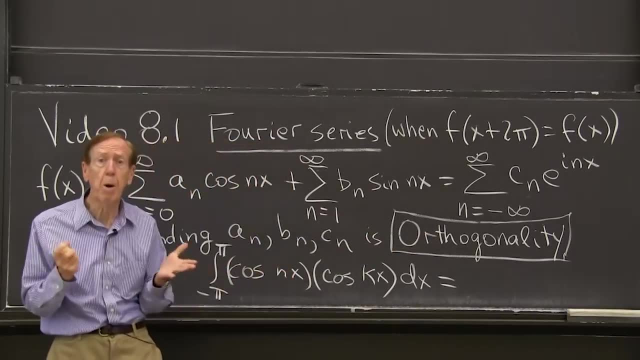 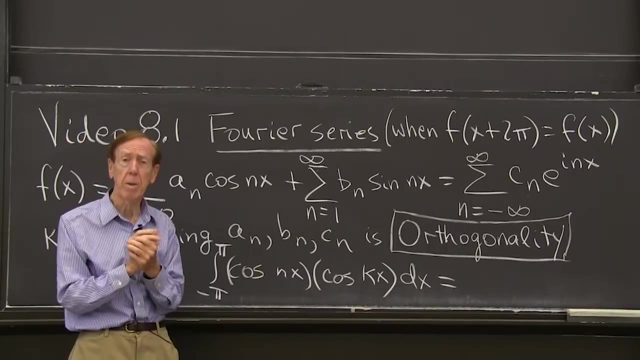 The key is orthogonality. So that's the first central idea here in Fourier series. It's the idea of orthogonality. Now what does that mean? That means perpendicular, And for a vector and a second vector we have an idea of what perpendicular means. 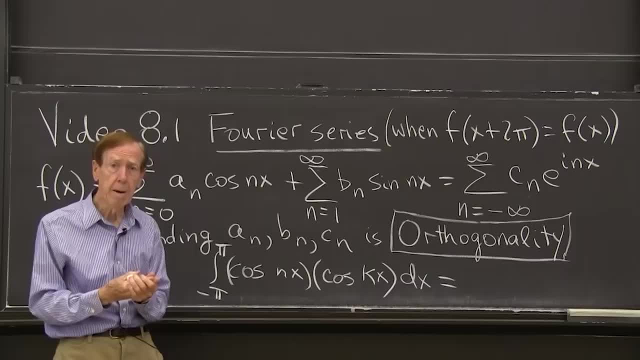 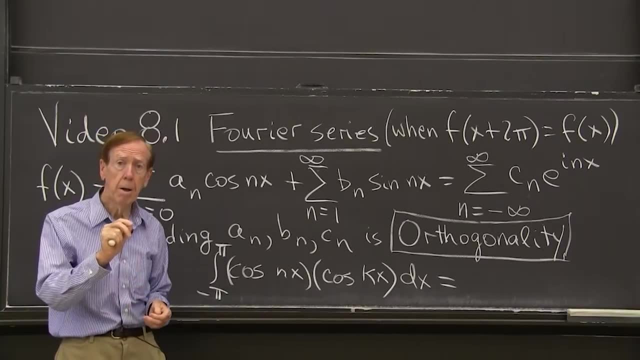 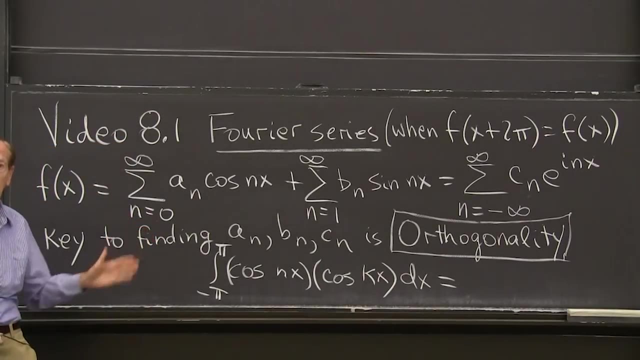 A 90 degree angle between them And we check that by the dot product or inner product, whichever name you like. between the two vectors should be 0.. OK, But here we have functions, So I have to say like cosine functions. 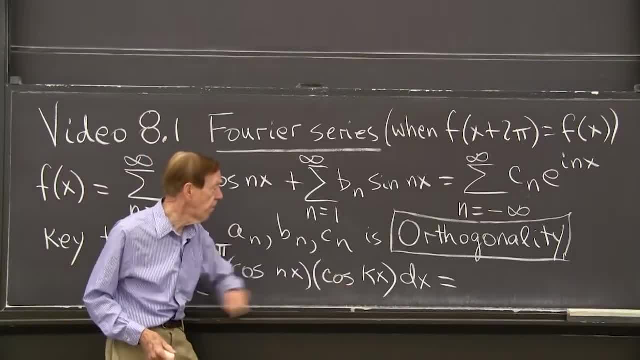 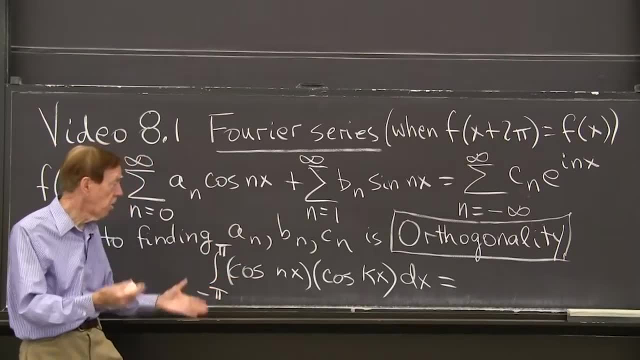 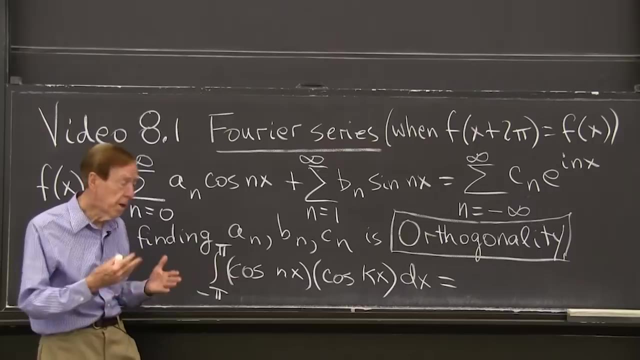 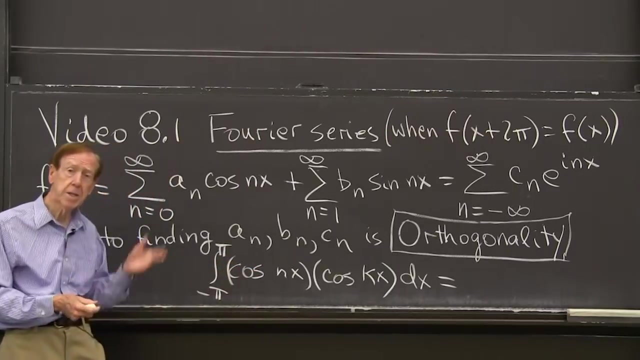 So here's one cosine and here's a different cosine. So those are two different basis functions, Say cosine of 7x and cosine of 12x. The coefficients a7 and a12 would tell us how much of cosine 7x is in the function. 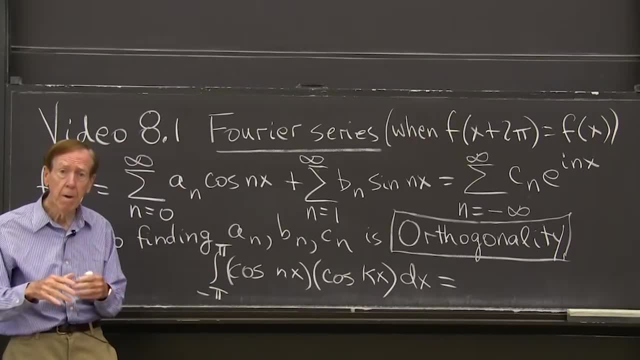 You see, we're separating the function into frequencies, We're looking into pure oscillations, pure harmonics, And we expect probably that the lower harmonics, the smoother ones, cos x, cos 2x, cos 3x. 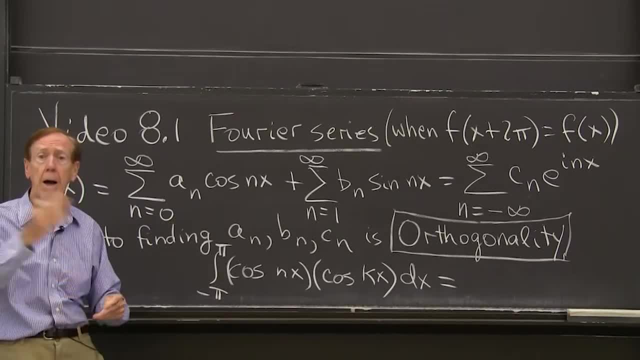 have most of the energy And the high harmonics- cosine 12x, cosine 100x probably. those are quickly alternating. Those contain noise and high frequency. Quick changes in the function will show up in the high frequencies. OK. 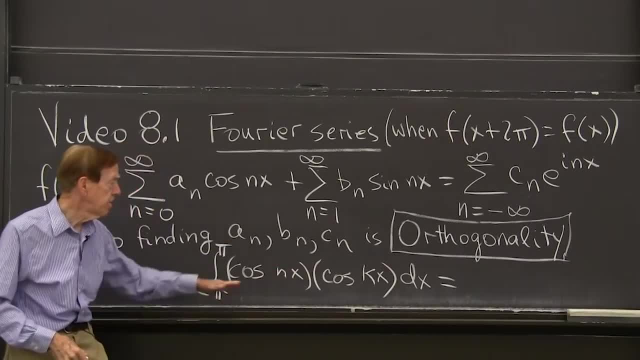 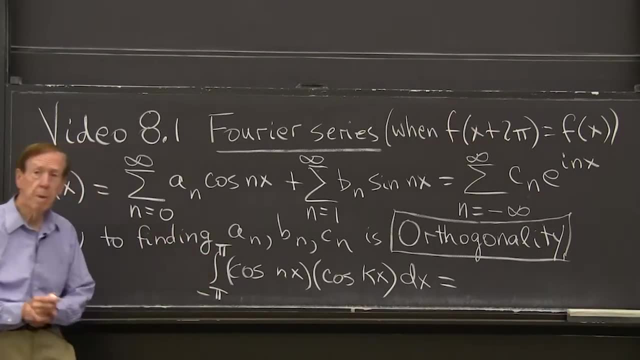 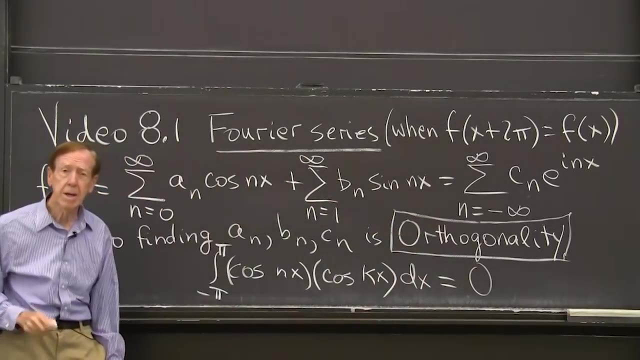 But now? so what's the answer to this integral Cosine of 7x times cosine of 12x dx over the range minus pi to pi? The answer is: orthogonality comes in. The answer is 0.. That's the crucial fact. 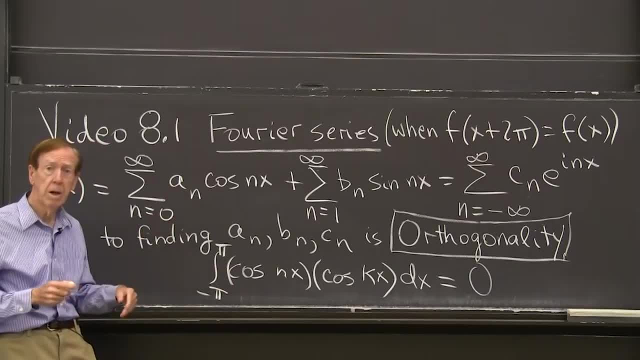 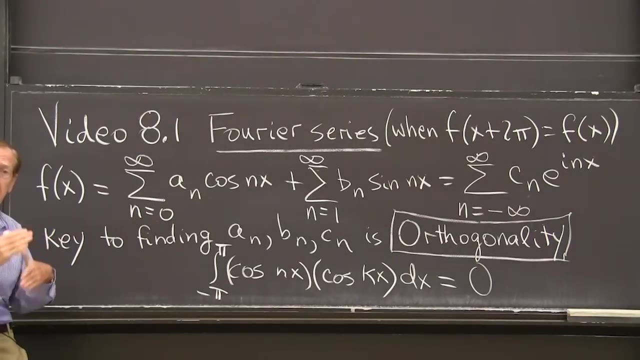 That's what makes it possible to separate out a7 and a12 and get hold of them. So let me show you how to do that. So I'm going to use this fact, which is the function version of 90 degree angle. So you see, it's a little like a dot product. 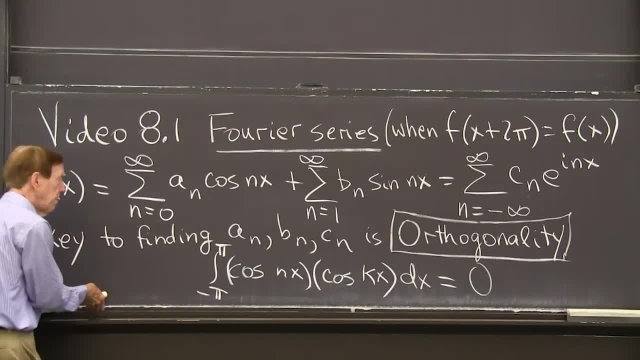 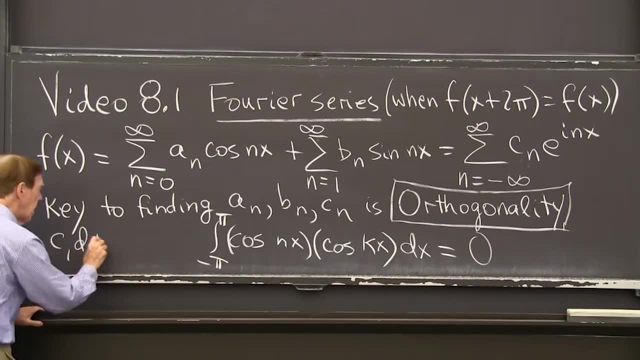 Dot product would. be well, let me remember, A dot product would be something like c1- d1 plus c2- d2 equals 0. If I had a vector c1- c2 and a vector d1- d2, that would be the dot product. 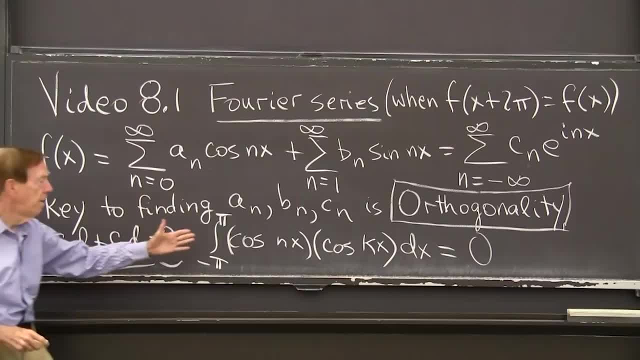 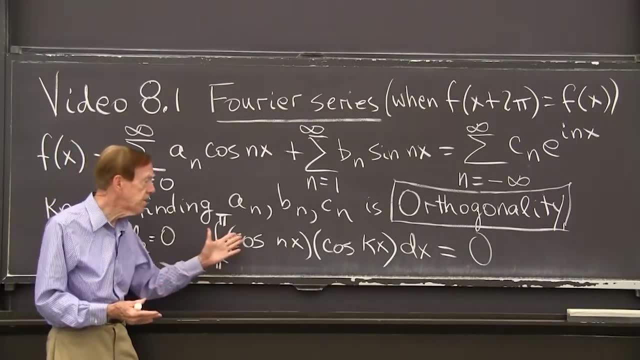 And it would be 0 if the vectors are orthogonal. Here, instead of adding, I'm integrating, because I have functions. So just that's the meaning of dot product: The integral of one function times the other function gives 0.. 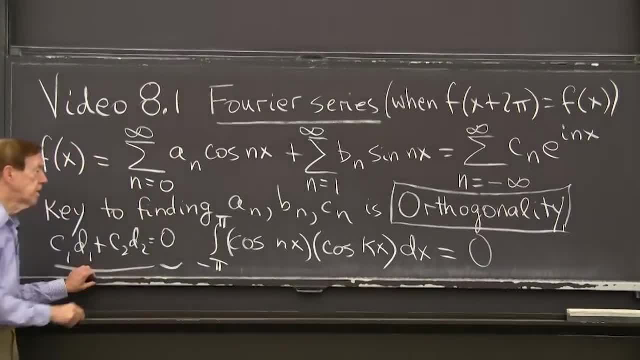 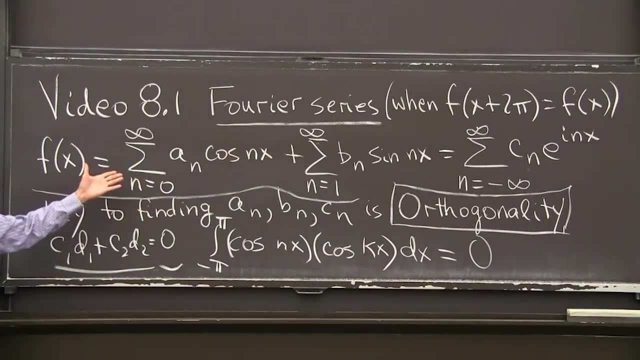 OK, I'll use that now. OK, how will I use this? I will look what I want. This is my goal. I'll multiply both sides by cosine kx. Multiply both sides of this equation by cosine kx, And then I'll integrate. 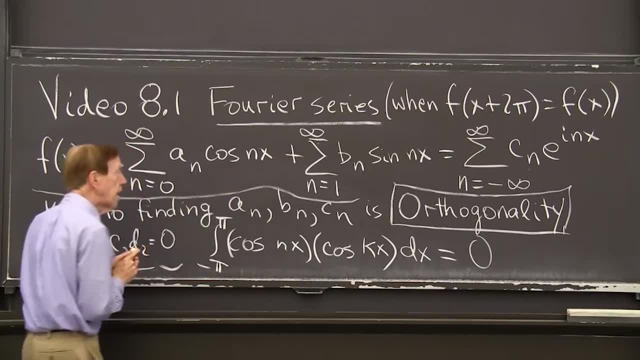 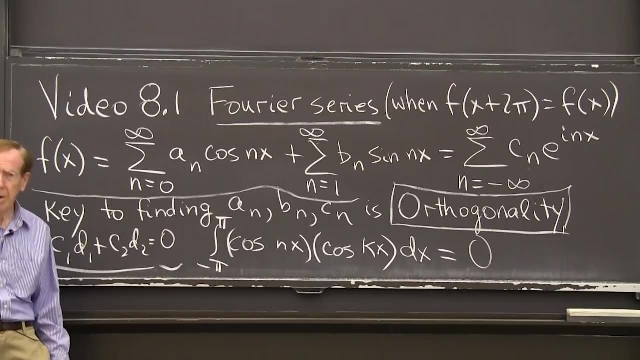 And the beauty is OK, That when I multiply by cosine kx and I integrate, everything goes to 0, except what I want. By the way, all the sines times cosine kx integrate to 0. All the sines are orthogonal to all the cosines. 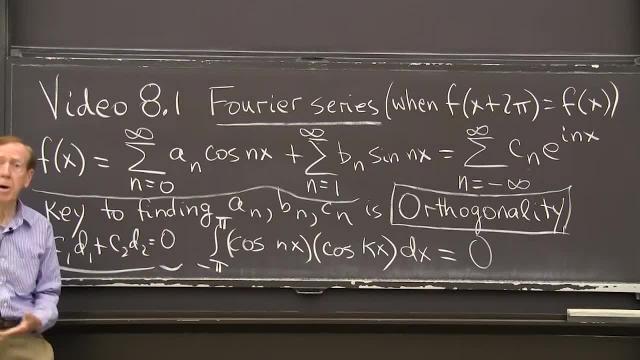 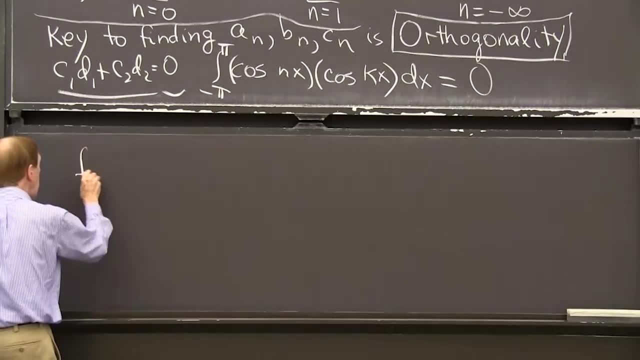 And all the cosines will be orthogonal to all the other cosines. So I'm only going to get. Let me show you what I get. So I multiply my f of x by cosine kx And I integrate from minus pi to pi. 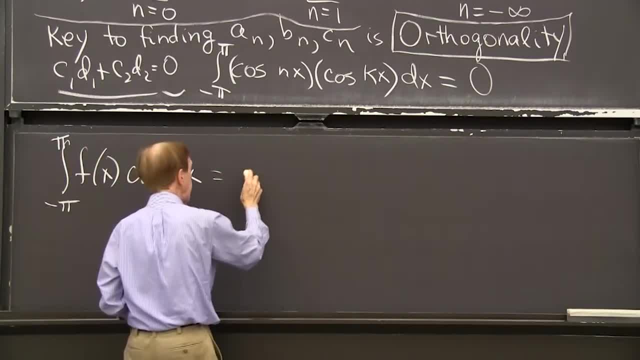 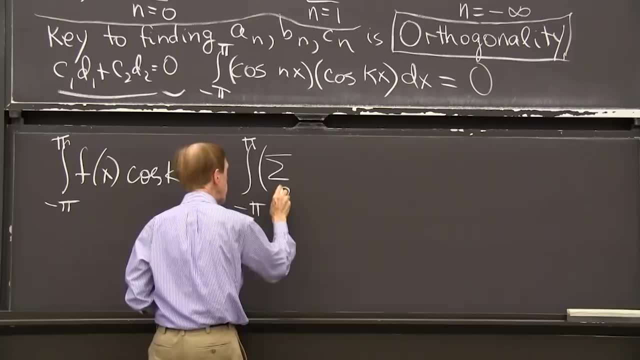 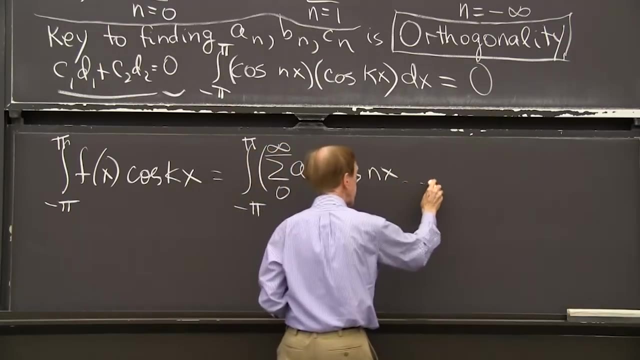 OK, now, on the right hand side, this is my integral, from minus pi to pi. Of my big sum of all these terms, 0 to infinity, a, n, cos, n, x, et cetera, including the sines, but I'm 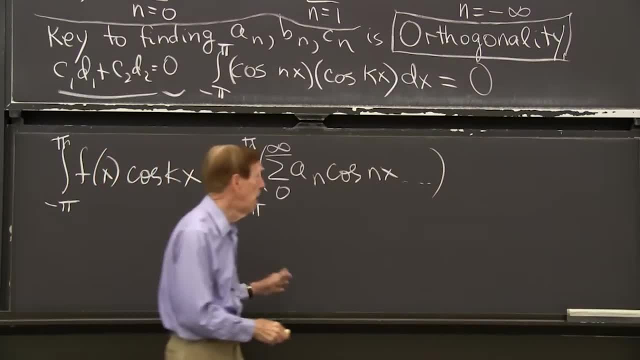 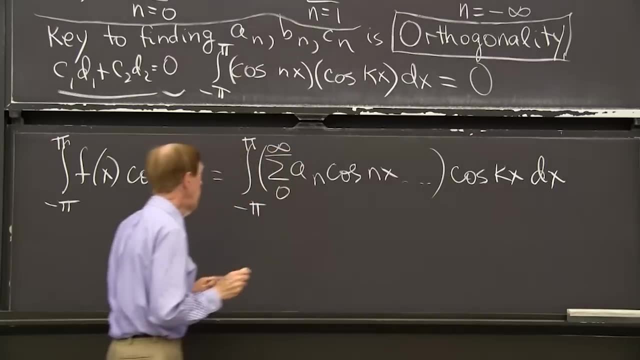 not even going to put them in because they're going to get killed by this integration Times. cosine kx- dx. All I did? All I did- was take the f of x, equal that formula multiplied both sides by cosine kx, and integrate. 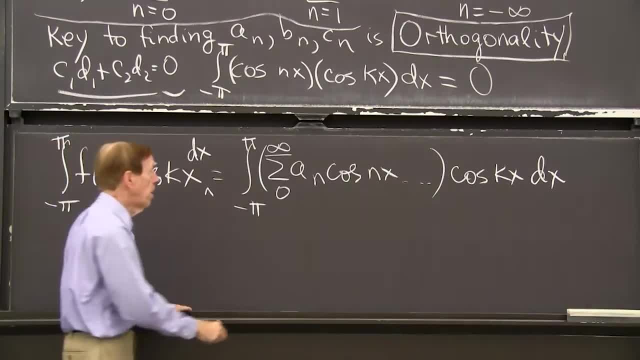 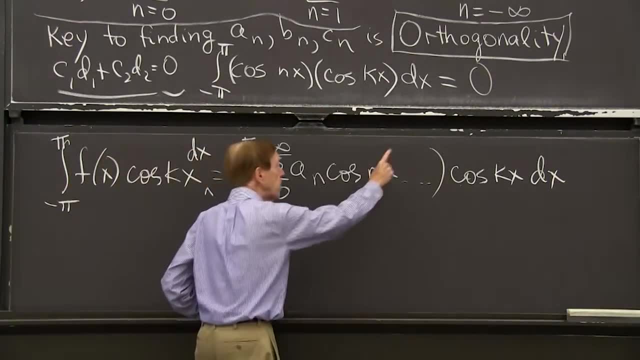 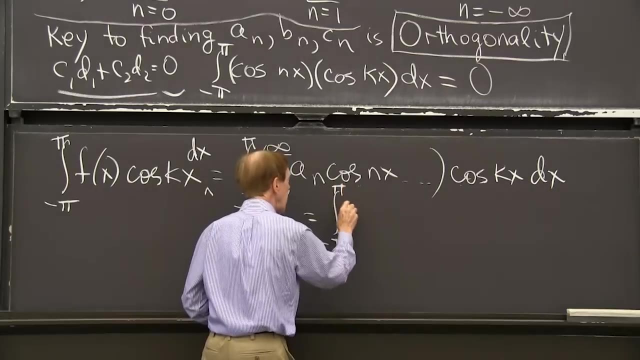 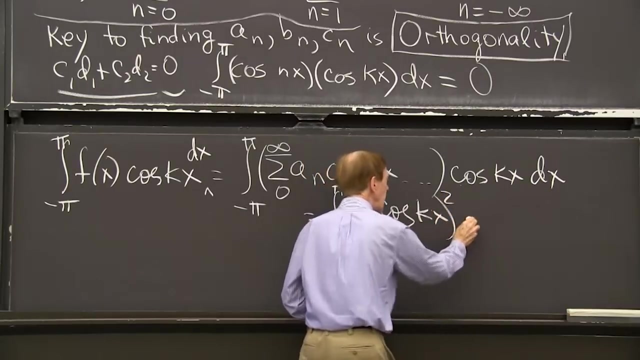 And now the orthogonality pays off, because this times this, when I integrate, gives 0. with one exception: When n equals k, then I do get the integral. The only term I get is ak, cosine, kx twice dx. Only k equal n survives this process. 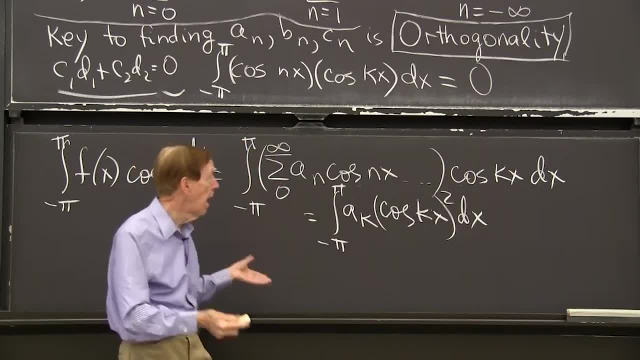 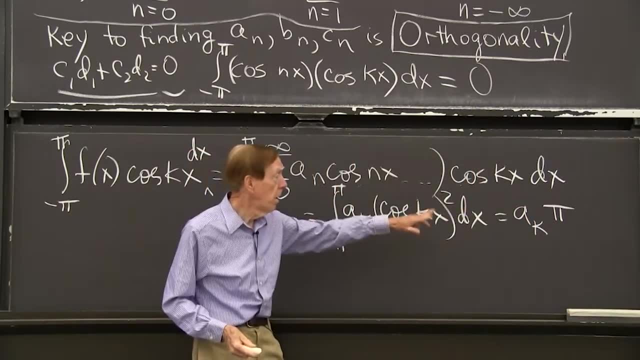 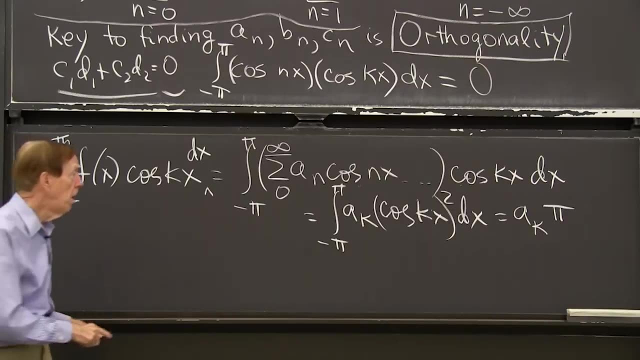 And then that integral of cosine squared happens to be pi. So this is just Just ak times pi. Look, I've discovered what ak is. I've discovered the k-th, Fourier cosine coefficient. I just divide by pi. So can I just divide by pi to get this formula for ak? 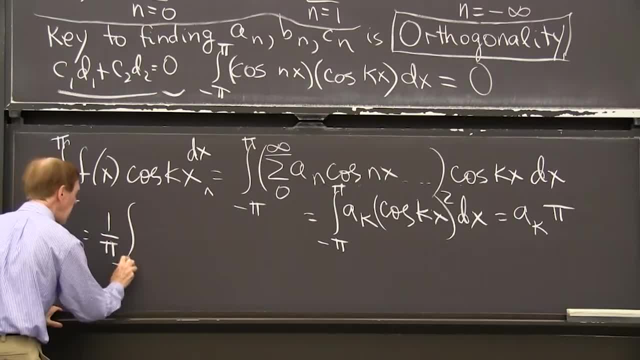 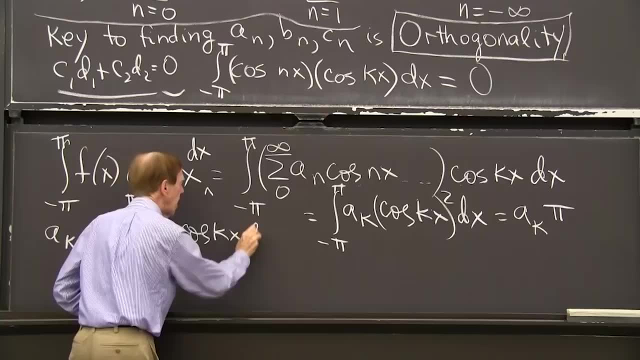 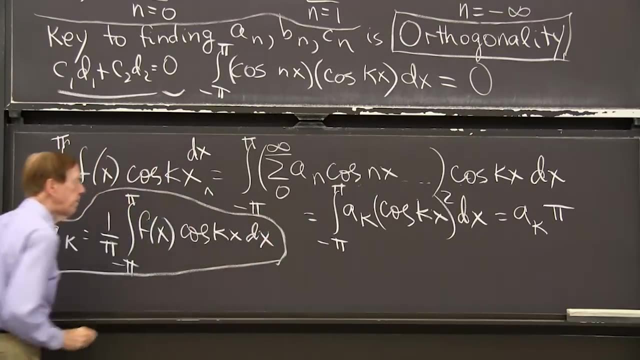 ak is 1 over pi, the integral from minus pi to pi of my function times, cosine kx, dx, dk, dk, dk. That's the formula That tells me the coefficients, And I could only do that with orthogonality. 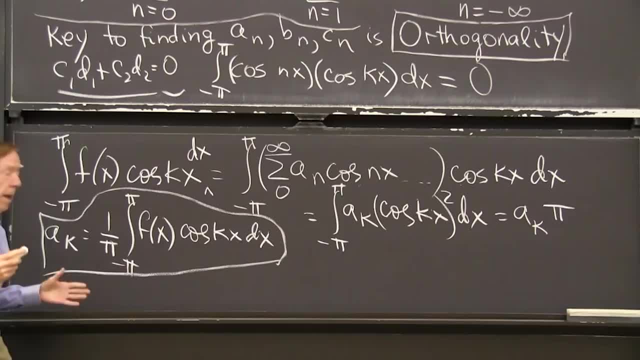 to knock out all but one term. And now, if I wanted to sine coefficients bk, it would be the same formula, except that would be a sine, Yeah. And if I wanted the complex coefficients, c, dk, bk. And now, if I wanted the complex coefficients. 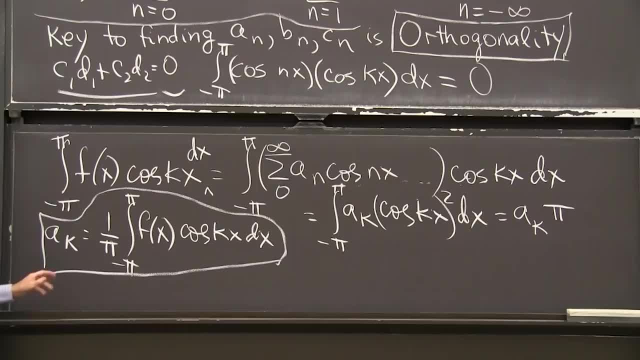 c, dk, bk. If I wanted the sine coefficients bk, bk, dk, dk. coefficient ck. it turns out it would be the same formula, except well, maybe it's 2 pi there, 1 over 2 pi. 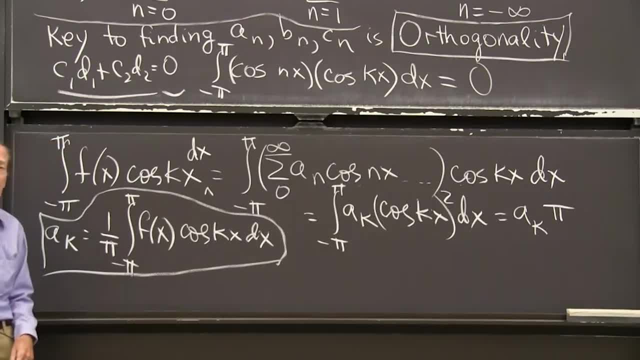 And this becomes an e to the minus ikx. In that complex case the complex conjugate e to the minus ikx shows up. So this is really the dot product, the inner product of the function with the cosine. OK, So let me do some examples. 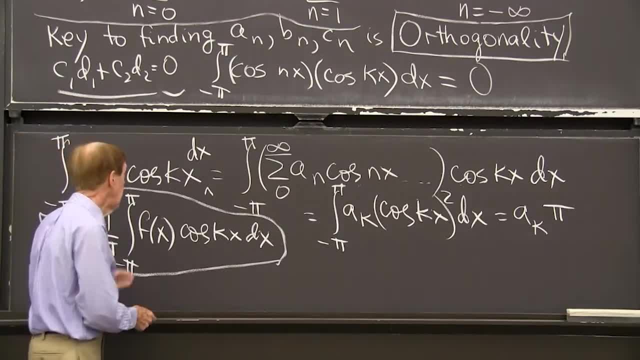 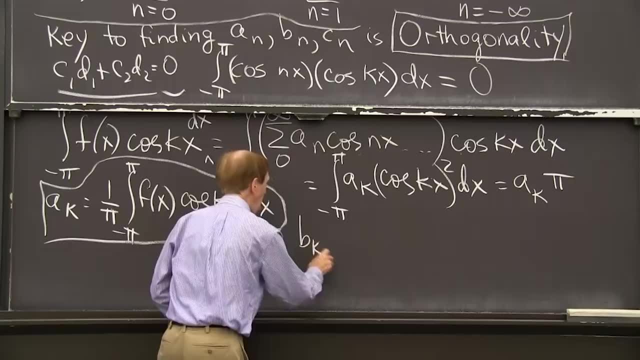 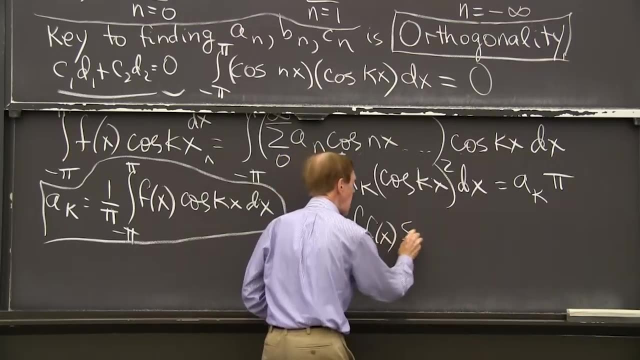 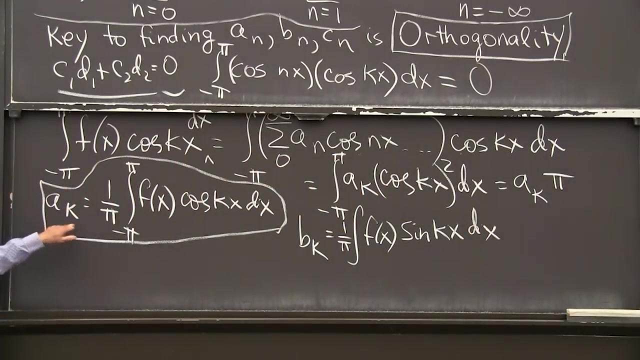 I'll start with one. Maybe I should write up the sine formula that I just mentioned. So bk is the integral 1 over pi, the integral of my function times sine kx, dx. And there's one exception. One exception, a0, has a little bit different formula. 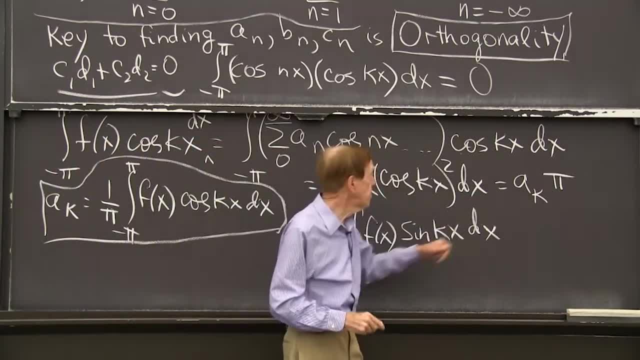 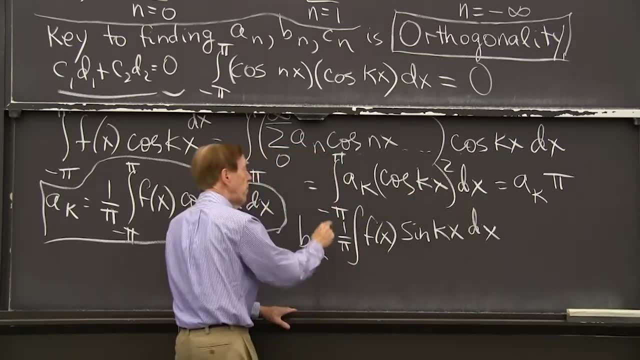 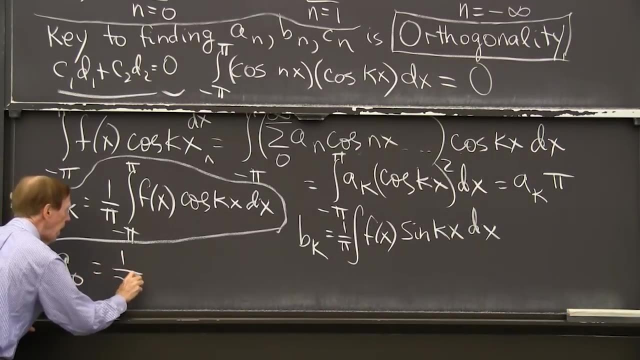 a0, the pi changes to 2 pi. I'm sorry about that. When k is 0, it's the integral of 1 from minus pi to pi and I get 2 pi. So a0 is 1 over 2 pi, the integral of f of x times. 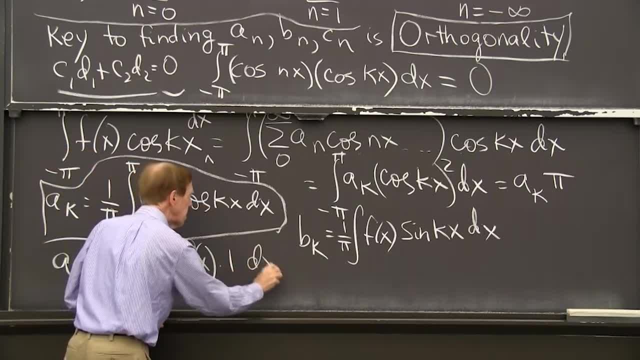 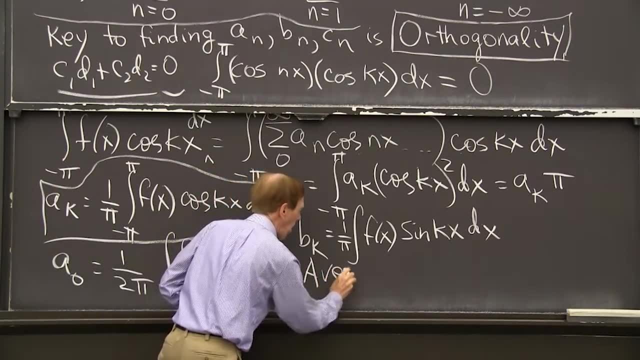 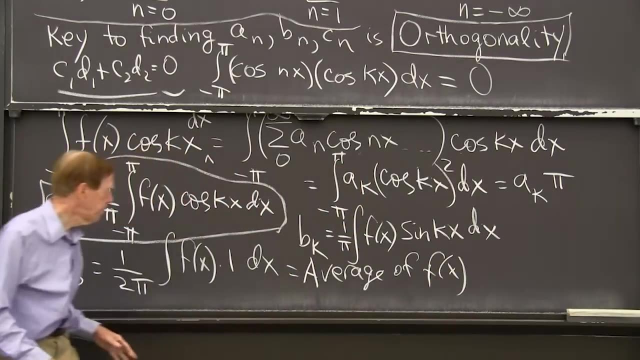 when k is 0,, cosine this is 1, dx. That has a simple meaning. That's the average of f of x, Right, OK? So the basis function was just 1 when k was 0.. When k is 0, the function, my cosine, is just 1.. 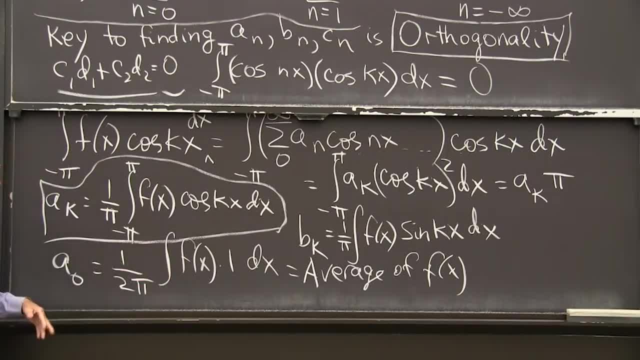 And I get the integral of the function times 1, divided by 2 pi. Could we just do an example? So I want to take a function And in this video, why don't I take an easy but very important function, the delta function? 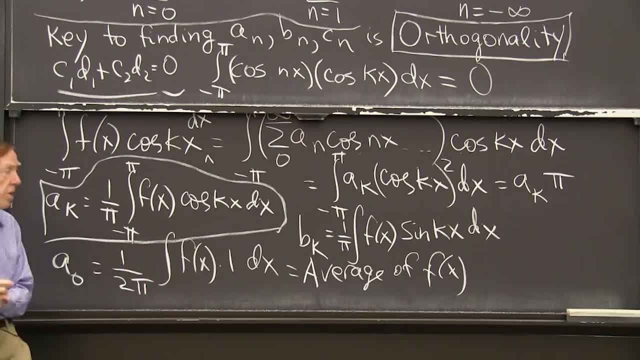 So I plan to use these formulas on the delta function. Let me draw a little picture of the delta function. I'm only going between minus pi and pi And the delta function, as we know, is 0.. It's infinite. Or. 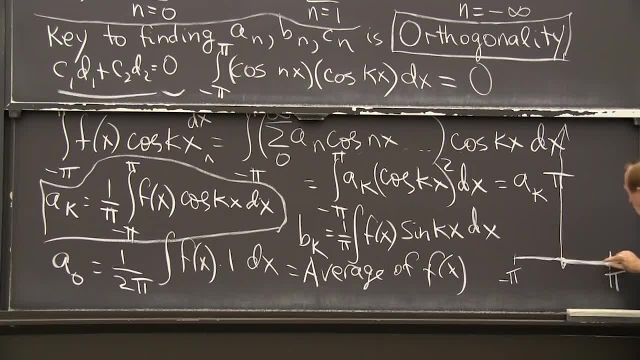 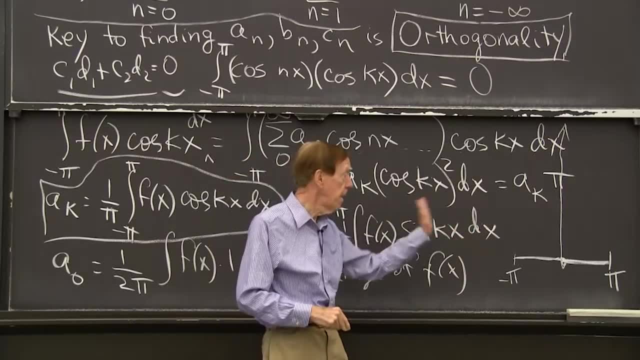 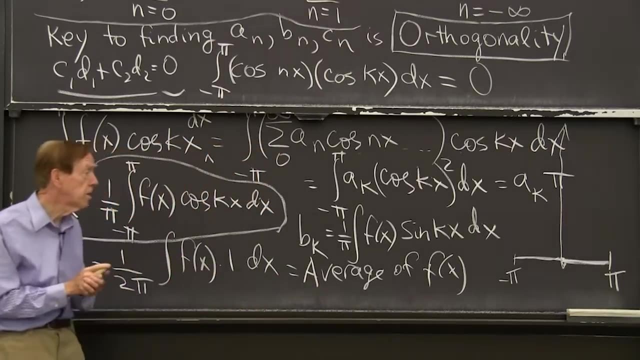 At the spike and 0 again. The reason I wanted to draw it is that's an even function, That's a function which is symmetric between x and minus x, And in that case there will be no sines. Sine functions are odd. 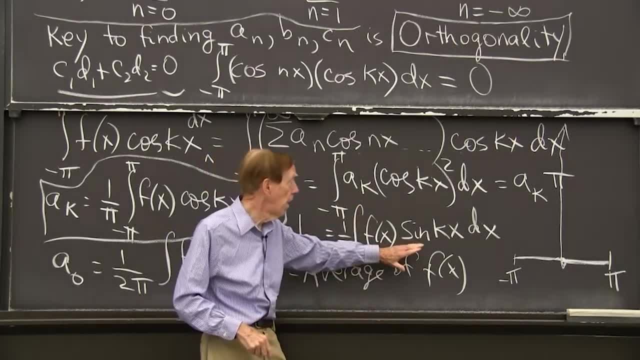 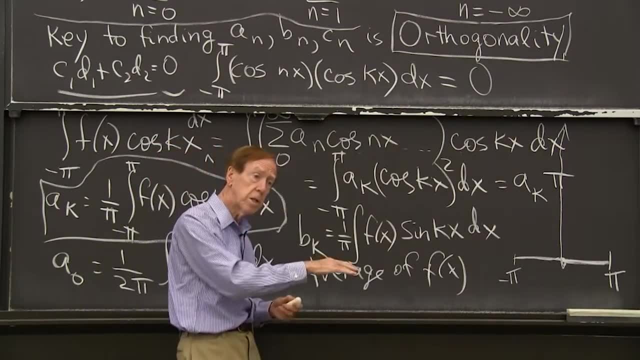 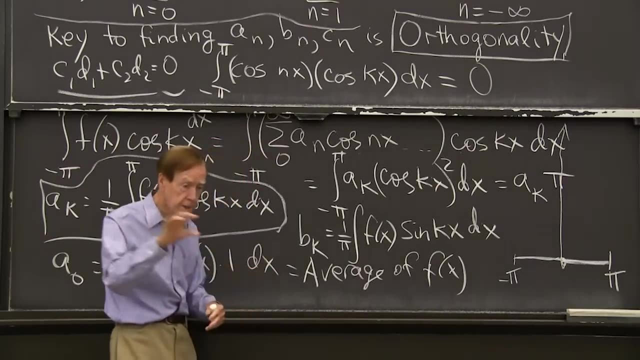 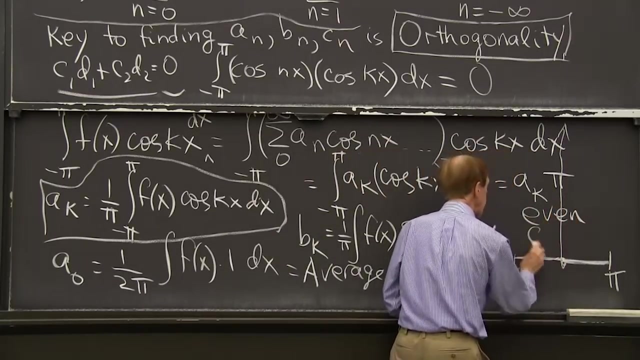 The integral from minus pi to pi of an odd function gives 0. The odd means that when you cross x equals 0, you get minus the result for x greater than 0. The point is this is an even function. Delta of x is the same as delta of minus x. 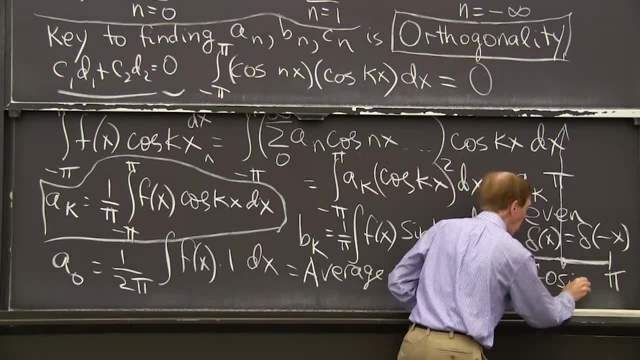 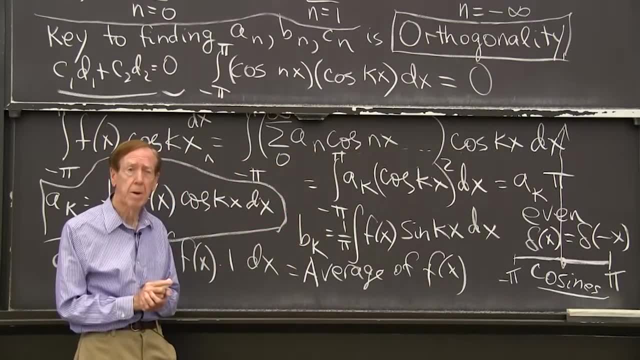 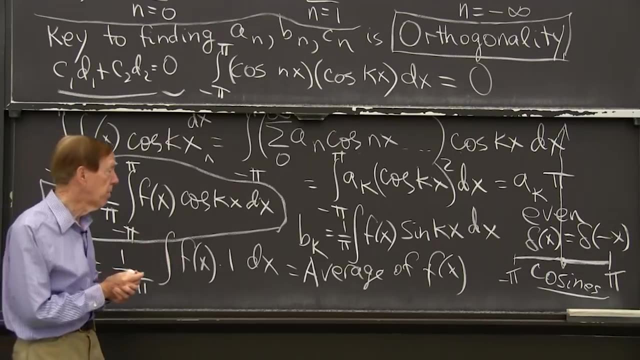 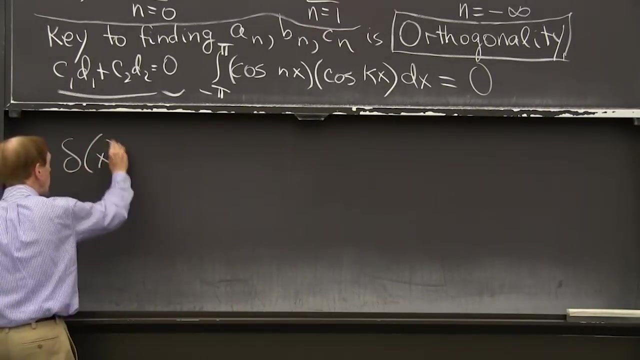 And only cosines. Good, The sine coefficients automatically are 0. So of course the integral would show it, But we see it even before we integrate. OK, I'm ready for the delta function, So I'm going to write delta of x. 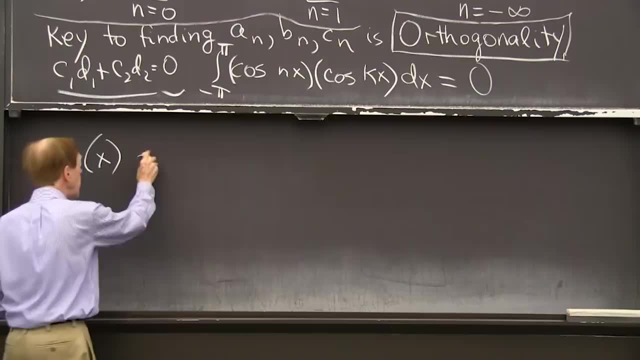 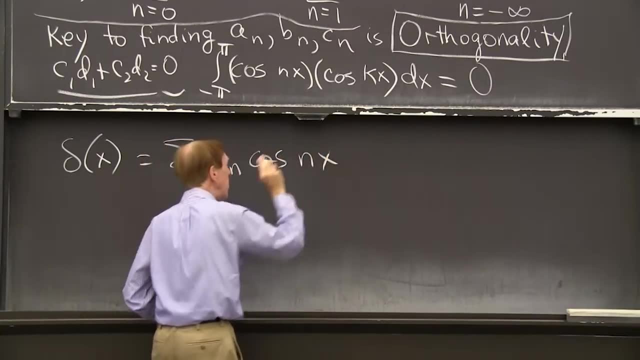 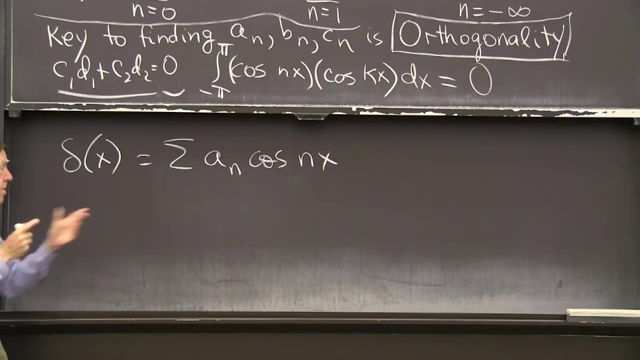 and we remember what the delta function is is a combination of cosines. OK, That's the delta function between minus pi and pi. OK, And what's our formula for the an? Well, you remember we had a special formula for a0. 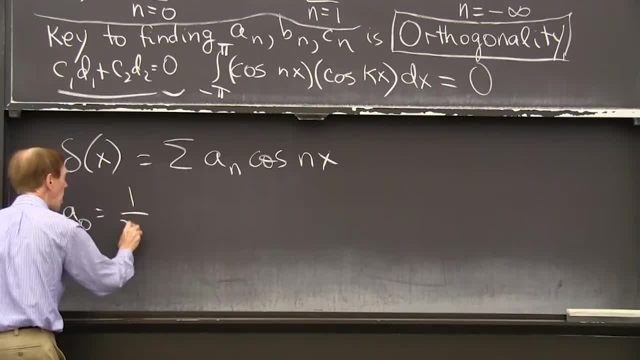 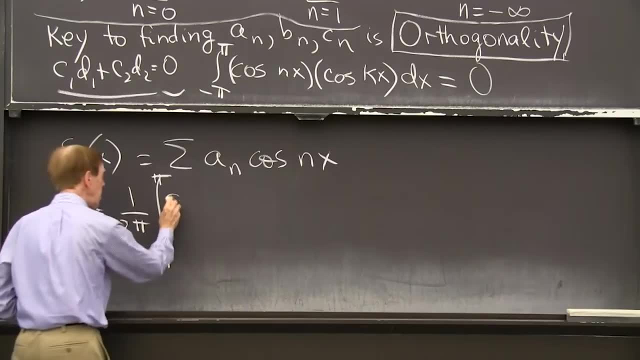 Which was 1 over 2 pi times the integral from minus pi to pi of our function, which is delta times the basis function, which n equals 0.. The basis function is 1 dx. OK, We know the answer to that. 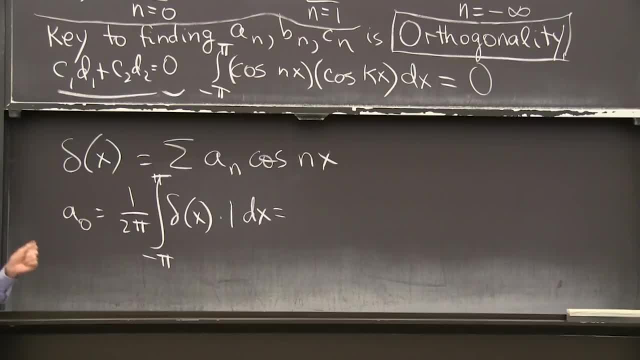 We can integrate the delta function. The one key thing about the integral of the delta function is it's always 1.. It's 1. if we cross x equals 0, which we will, So that integral is 1, so I'm getting 1 over 2 pi. 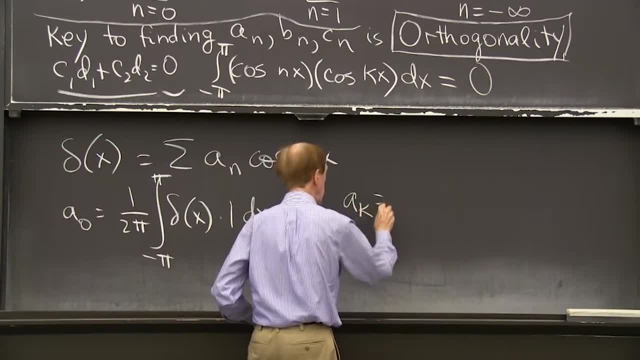 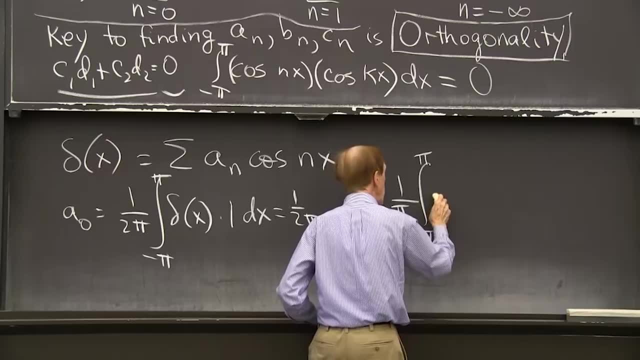 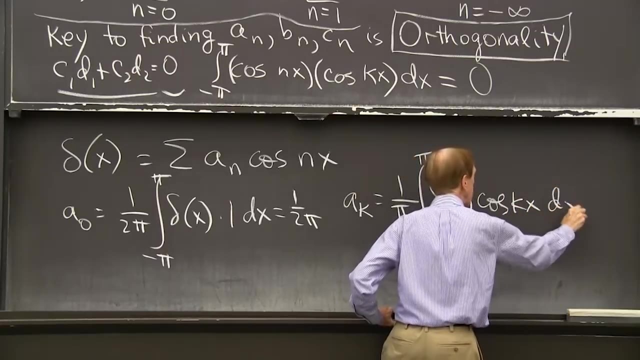 What about the other Fourier coefficients? So that's 1 over pi, now the integral from minus pi to pi of the delta of my function times, cosine, kx, dx. You know what I'm doing. I'm using my formula to find the coefficients. 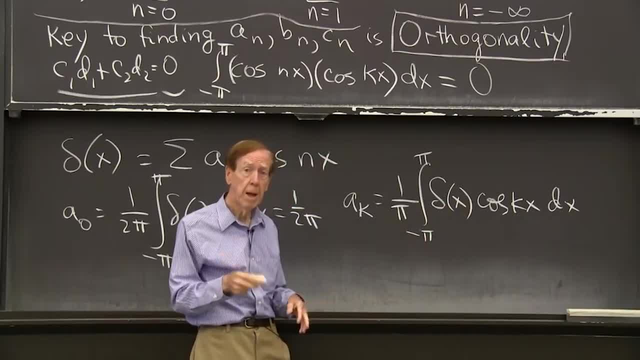 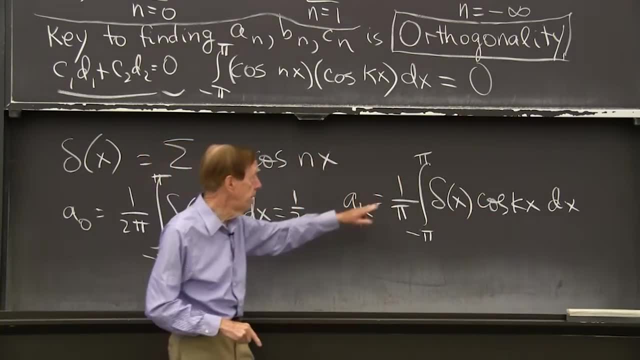 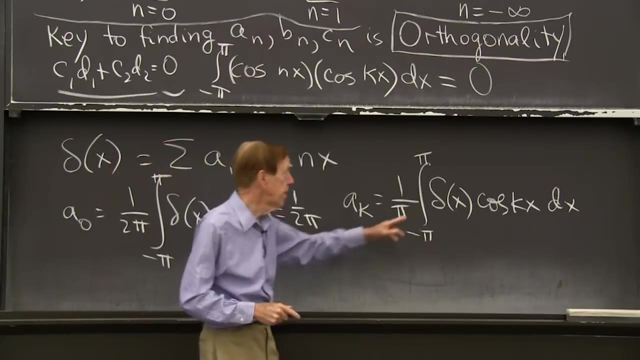 My formula says: take the function whatever it is- And in this example it's the delta function- Multiply by the cosine, integrate and divide by the factor pi. OK, Well, of course we can do that integral, Because when you integrate a delta function times, 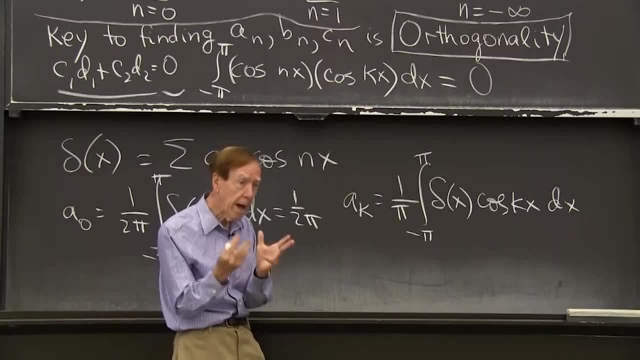 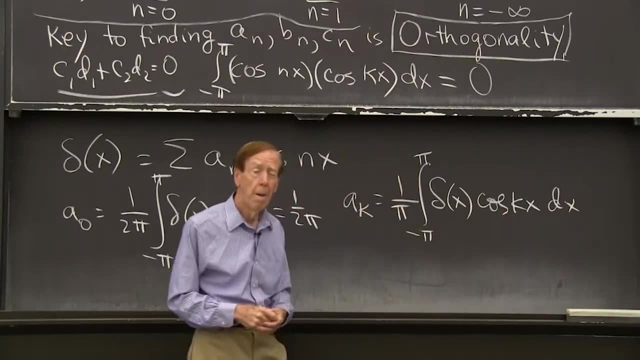 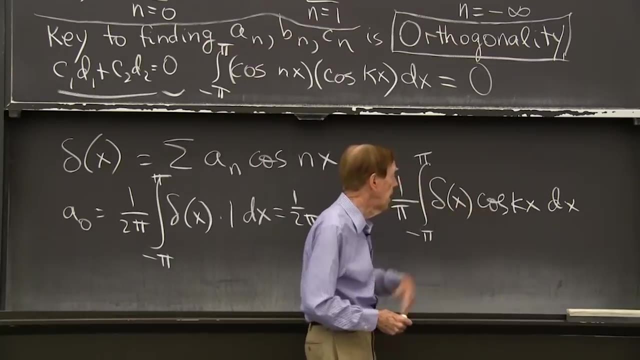 some other function you only get all the action is: at x equals 0.. At x equals 0,. this function is 1. And I don't care what it is elsewhere, It's just 1.. So this is the same as integrating delta of x times 1,. 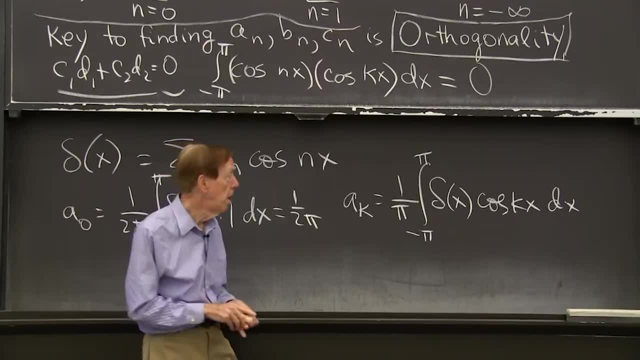 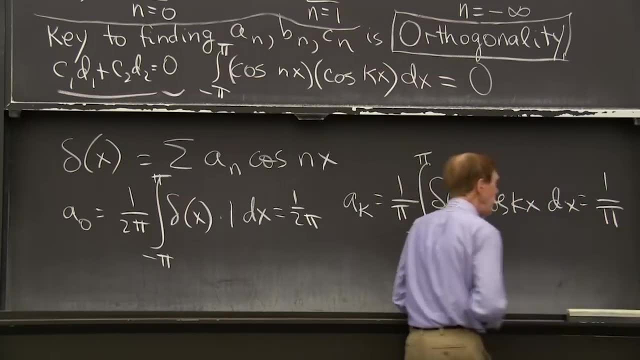 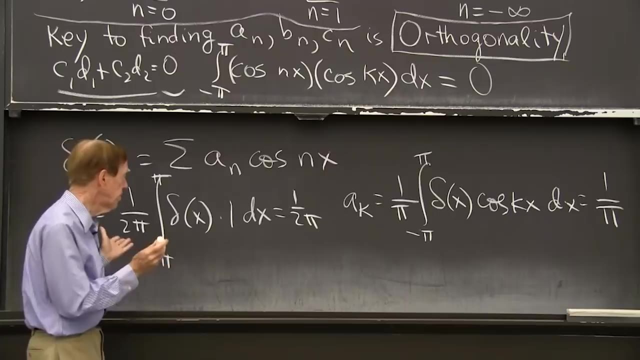 which gives us the integral of the delta function is 1.. So this gives us that integral is 1.. So I'm getting 1 over pi. Good, OK. So now do you want me just to write out the series for the delta function?